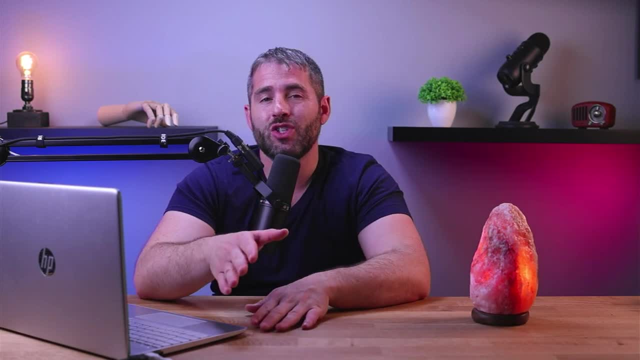 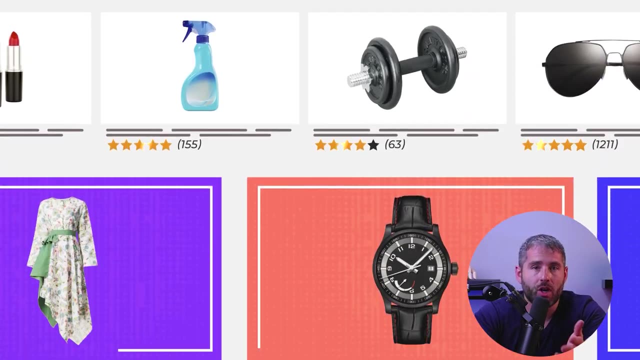 to run your website, as well as the scalability of the web hosting solution to allow for future growth. On top of that, you should consider the level of security required for your website, such as in the case of an online store that needs to protect customer data. 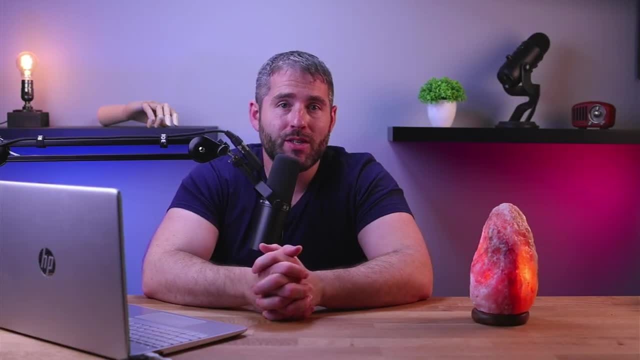 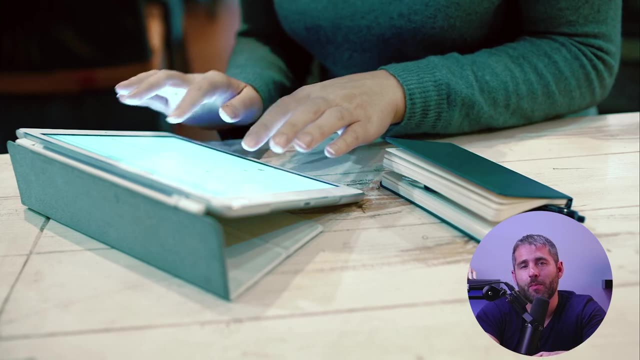 Finally, setting up a budget for your hosting services can help organize your long term spending. By understanding these factors, you can make better decisions in your search for the right web host, and it's recommended to write down your website needs before proceeding. Once you're done with that, you're going to need to research and compare sites. 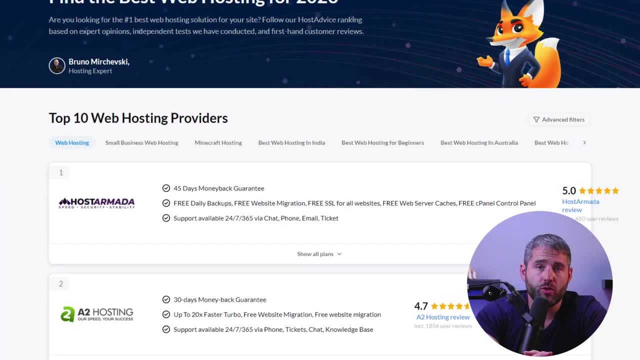 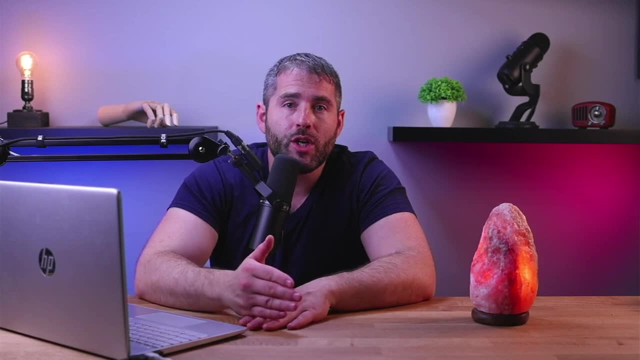 And here's some tips on how to do that. First, check out reviews from real users on sites like HostAdvice and Trustpilot. These platforms are known for providing honest and impartial feedback, which will give you a good idea of what you can expect from the provider. 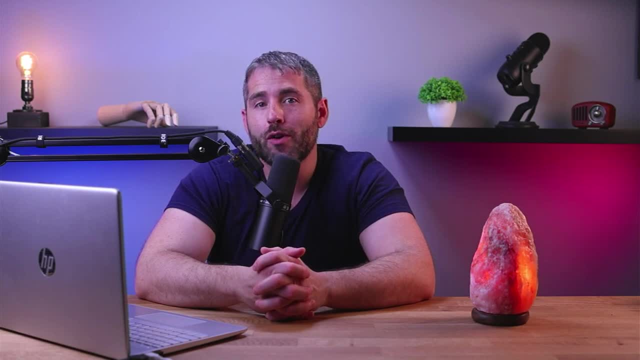 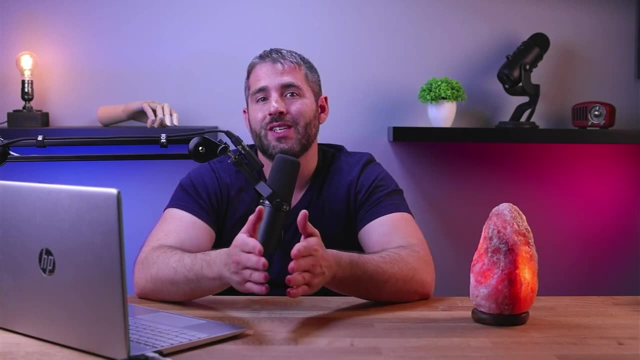 Another way to assess a hosting provider's legitimacy is to look for money back guarantees or free trial options. This will help you to try out the web host services without risking any of your hard earned cash. Finally, it's always a good idea to contact customer support. 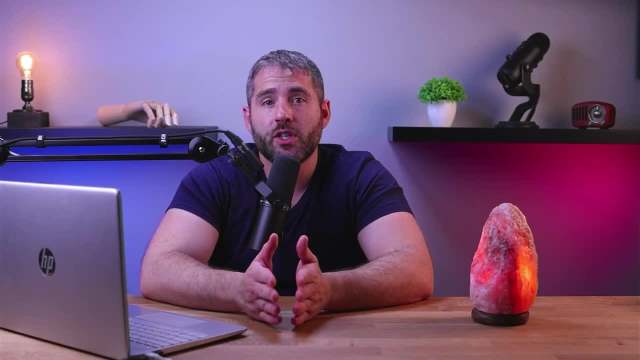 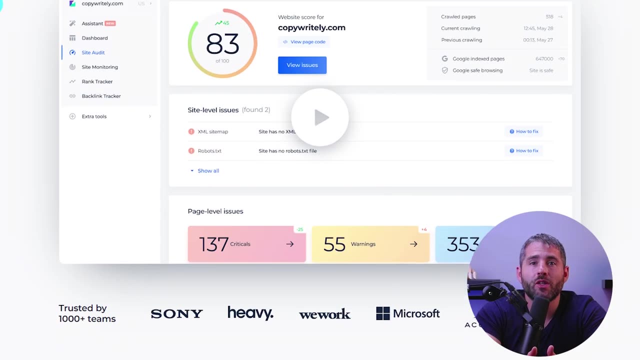 and see how responsive they are. If a provider takes a long time to respond to customer queries or doesn't provide helpful solutions, it might be best to steer clear. If you want to take things a step further, you can use online tools like Site Checker to reveal a website's hosting provider. 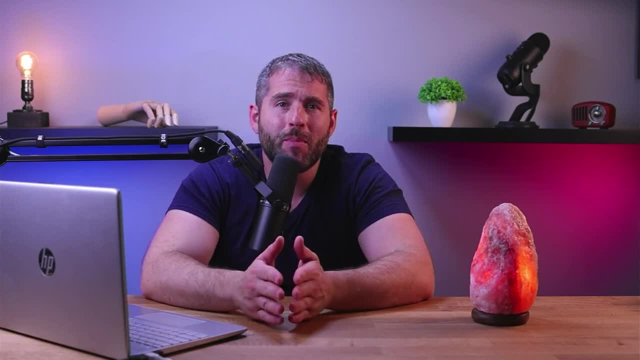 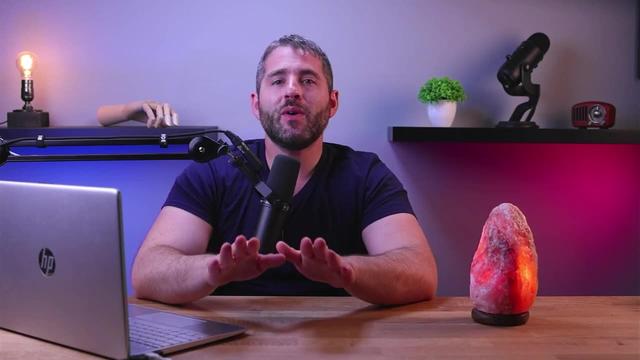 This will give you a clearer idea of which providers are most popular and might be worth investigating further. We recommend making a list of your top three providers so you can easily compare their pros and cons. Now it's time to compare their technology and features to determine which one is the best fit for you. 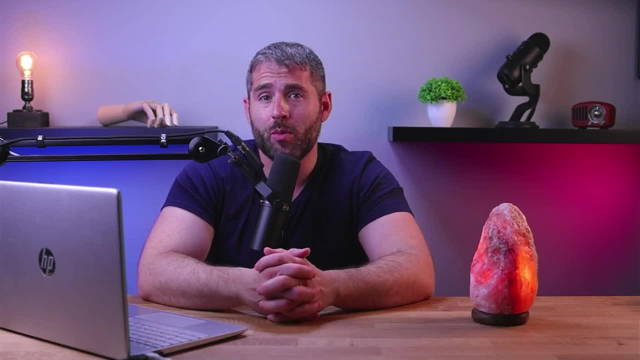 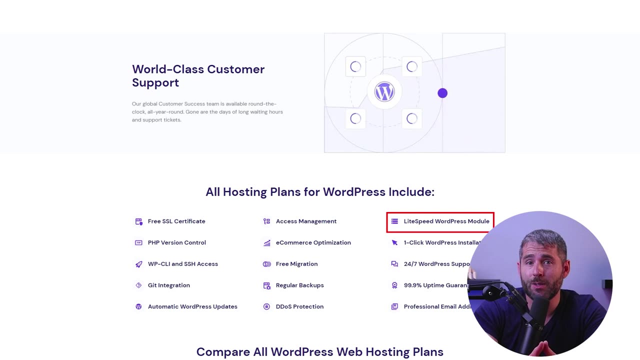 Each hosting provider has its own unique approach to boosting website performance, so it's important to do some research before making a decision. For example, Hostinger, which is a service I personally use, has Lightspeed Web Servers, LSWS and an in-house web application firewall. 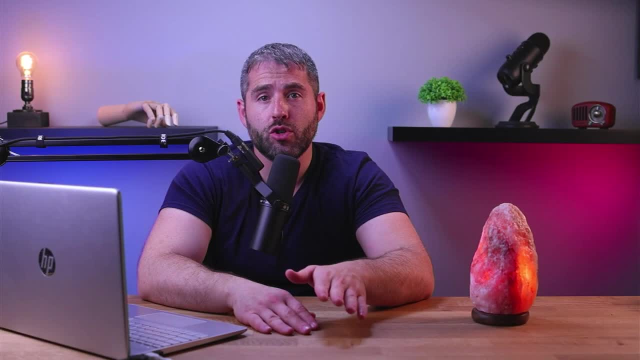 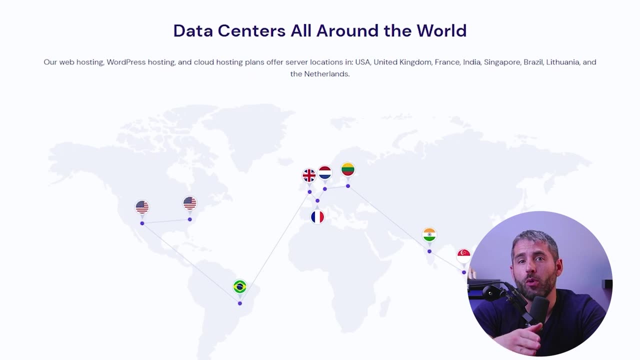 to enhance its technology and strengthen security. As you continue your search, here are a few factors to keep in mind. Firstly, check out the web host data center. It's a good idea to choose a provider with multiple server locations worldwide and make sure there's a data center near you to ensure low latency. 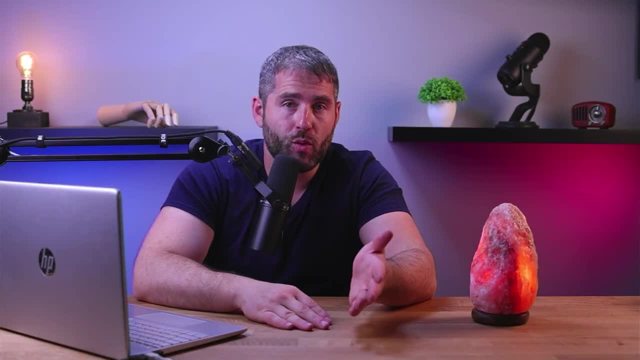 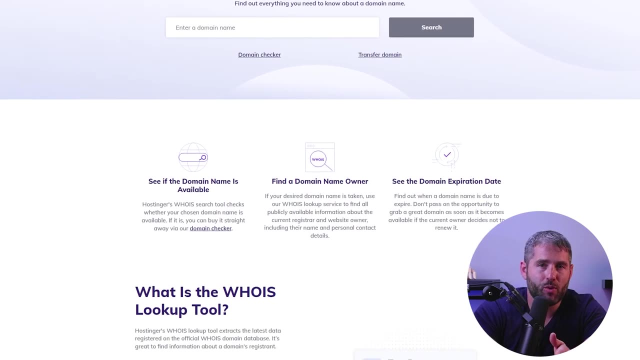 Next, see if the provider offers a migration option. if you're looking to transfer web hosts, Hostinger, for example, offers a free and seamless website migration service. Domain names are also a crucial element of a website, so check if your web host offers. 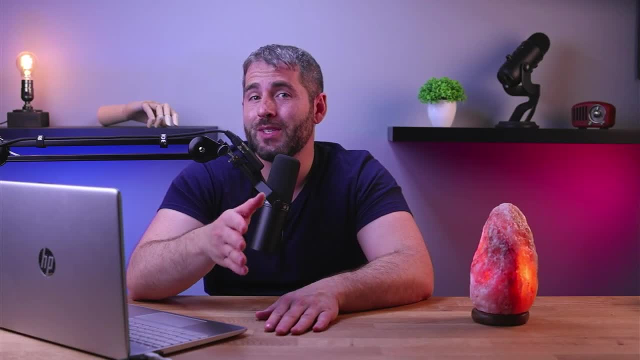 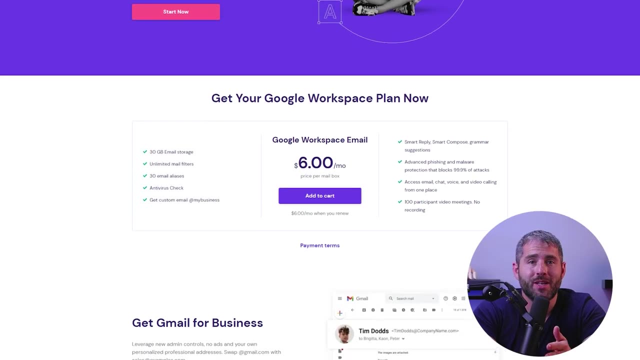 domain name registration with their hosting plans. This can simplify the website building process and help you choose the right domain for your site. Finally, having a custom email is a great additional feature. It can help boost your credibility, so keep an eye out for web hosts that offer email. 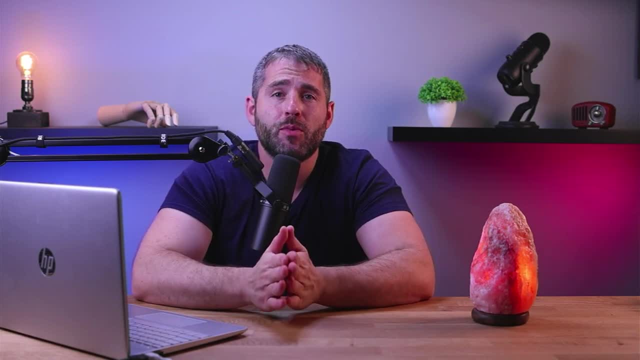 services Moving on, it's extremely important to have a dependable support team that can help you out any time, day or night, to fix any website issues that may come up. Before picking a web host, it's essential to ensure that they offer various support. 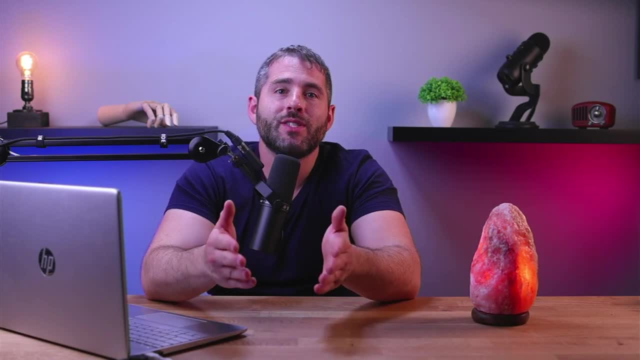 options. There are different types of support services, but here are some of the main ones you should look for when selecting a web host. Live chat is a popular customer service method that's ideal for getting feedback. Live chat is a popular customer service method that's ideal for getting feedback. 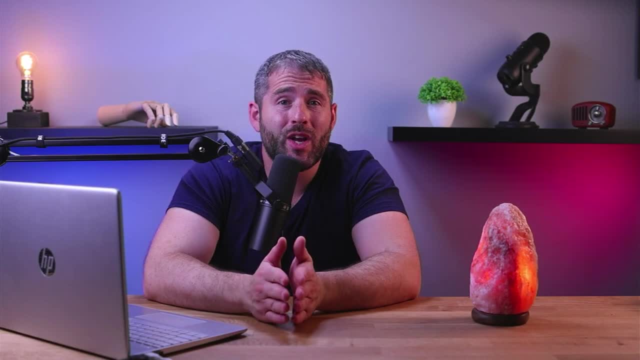 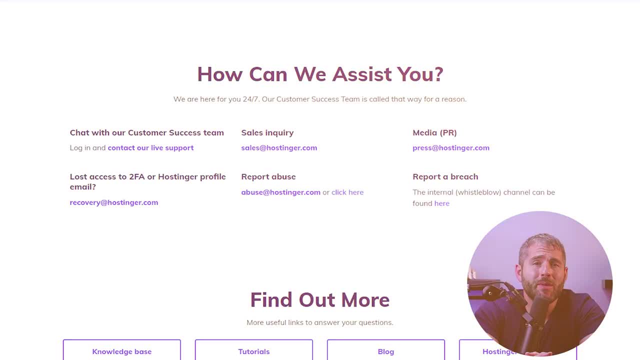 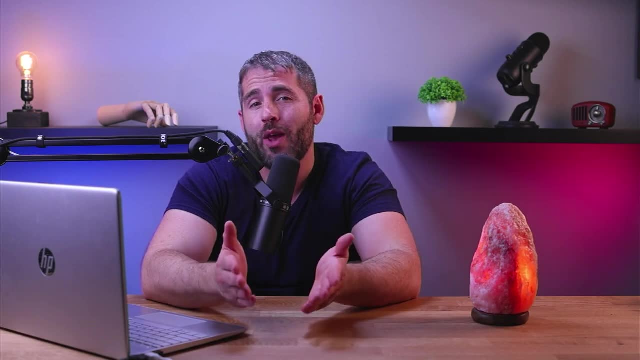 Most web hosts also provide transcripts of the conversation to keep track of problems and progress. Email support is also an excellent option for non-urgent issues or enquiries. Customer service can solve the problem without responding right away. It's Assaltet Web Hosting. A Seminal Set up web hosting. you're probably 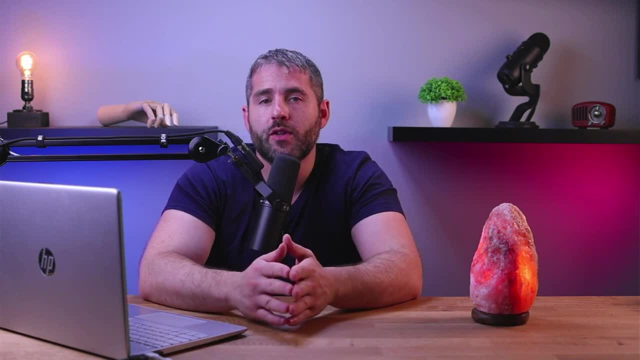 Jumping from object to object. what's this? Head on over to bitcom. there are a variety of standard web hosting Shop and I tell you the cookies in the pro server have changed over time. Again, doing ads to goodus is a key factor when you look for the actual bed room desk. 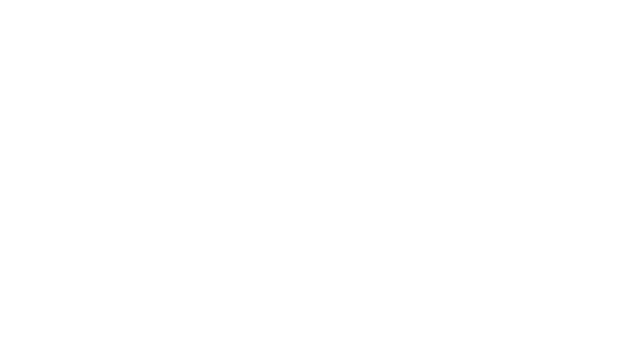 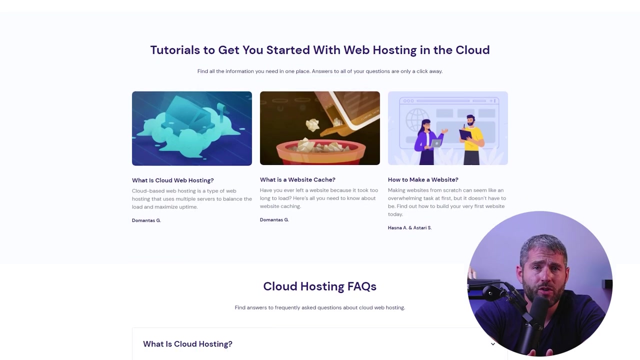 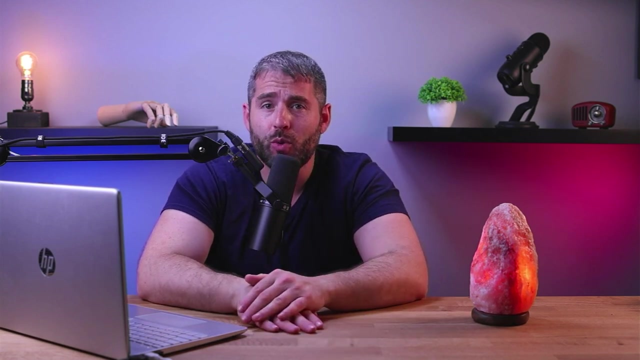 app knowledge base that answers frequently asked questions. This resource can be particularly helpful for beginners in website development. A reliable web host will provide industry-related tutorials and blog posts. This is excellent for people who like to learn and solve problems independently. If you're unsure about a provider's customer support quality, you can check reviews about. 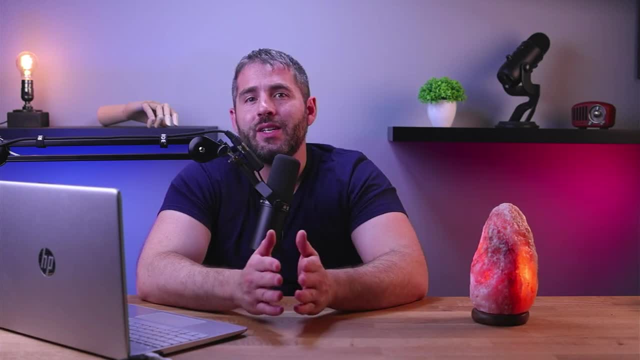 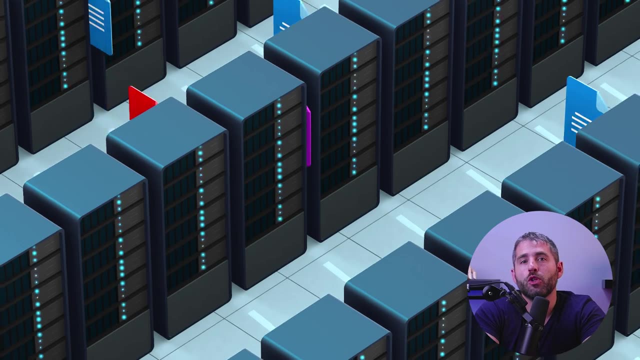 their service. Next, you're going to need to find the right hosting plan Now. there are many different types of hosting services available, and each one has its own pros and cons. First, we have shared hosting that allows multiple websites to run on the same physical. 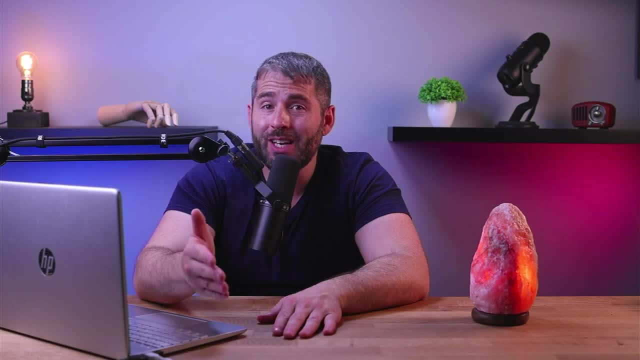 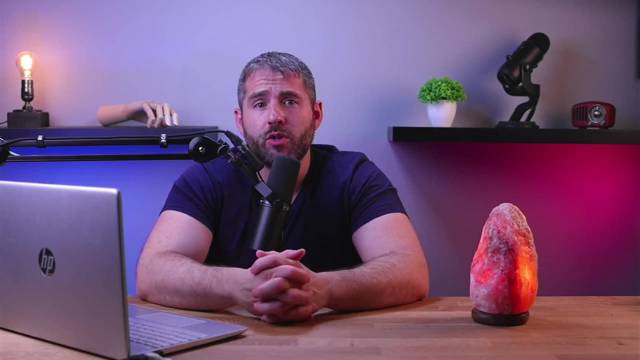 server and share its resources, which means that any issues faced by other websites on the same server can affect the performance of your own site. Compared to other types of hosting, shared hosting is the most affordable and requires minimal technical knowledge. Most shared hosting providers offer a user-friendly control panel that simplifies website management. 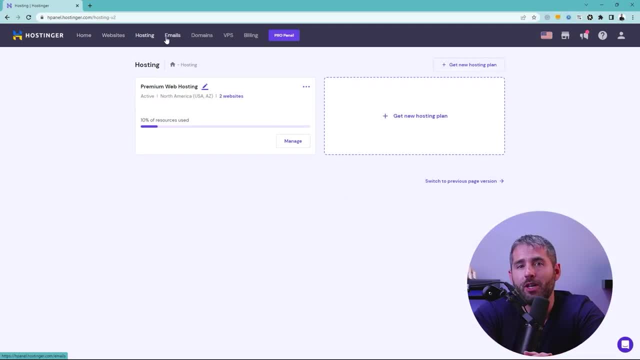 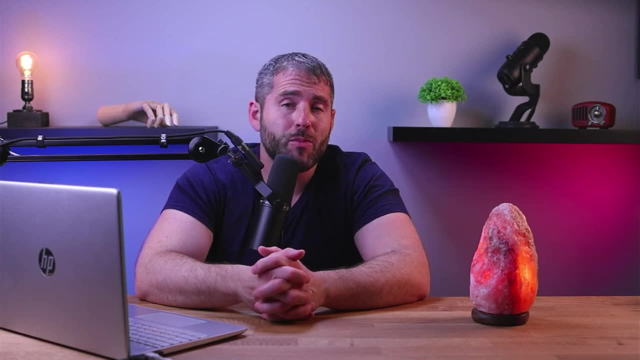 Hostinger, for instance, has an intuitive custom H panel that makes website management a breeze. Shared hosting is ideal for low to medium traffic Hosting is also ideal for small business sites such as personal portfolios and blogs. Another hosting option is VPS hosting. 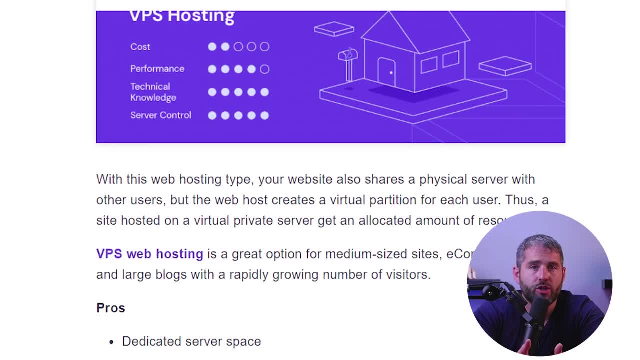 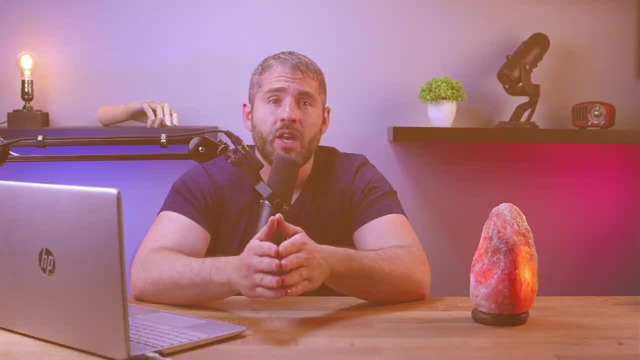 VPS, or virtual private server hosting, provides you with a shared server, but with dedicated partitions that guarantee more stable and secure website performance thanks to allocated resources. It's crucial to consider the compatibility of your preferred operating system when selecting a VPS hosting plan. 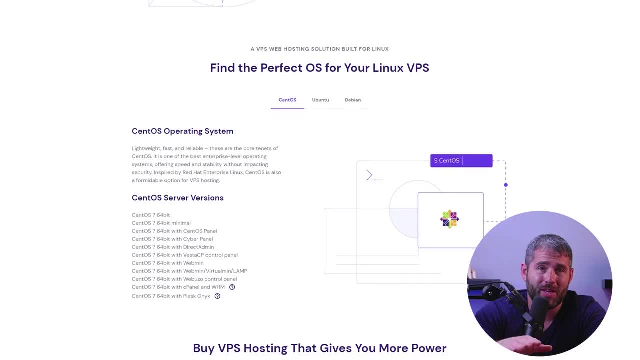 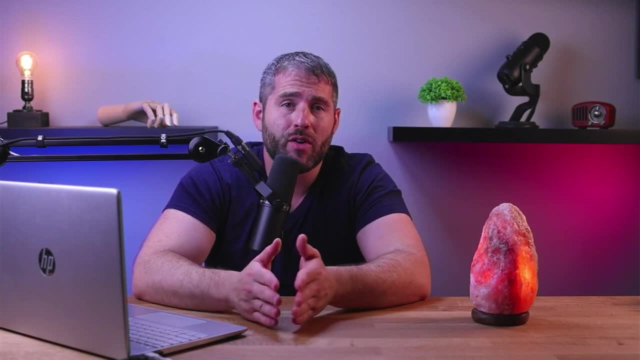 For example, Hostinger offers instant Linux deployment for their VPS plans. VPS hosting is an excellent option for medium-sized sites. Hostinger is a medium-sized website, since it's a middle ground between a shared and dedicated server. However, it requires technical expertise and has a steep learning curve, since site owners 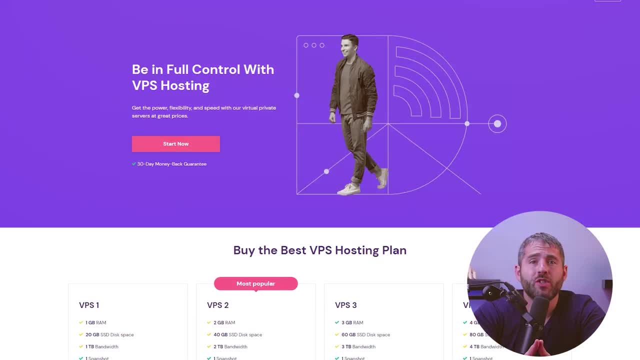 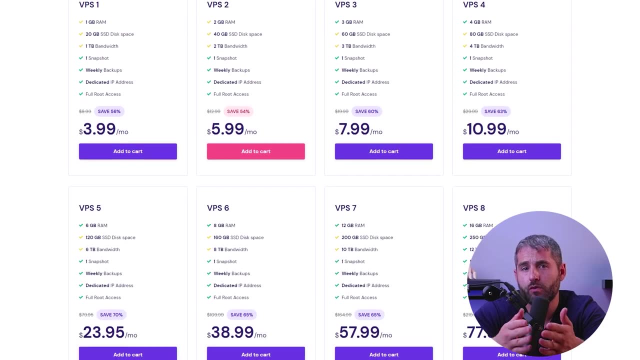 get full root access to configure and maintain the server. Hostinger offers 8 VPS plans that vary based on memory, storage space and bandwidth, allowing you to choose the most appropriate VPS for your project. Next up, we have Cloud Hosting. 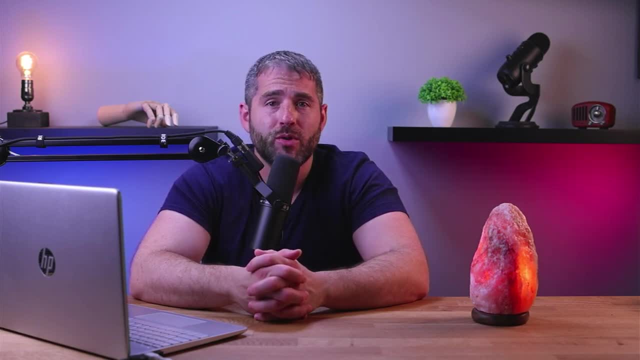 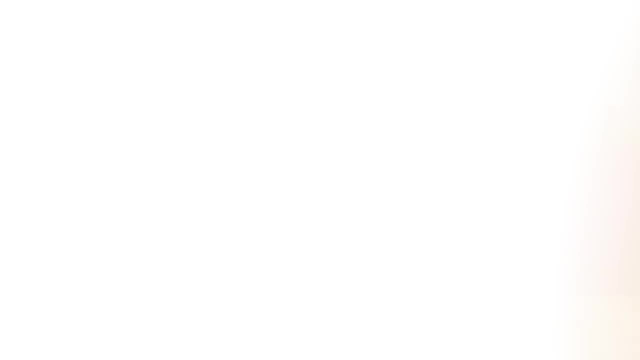 Cloud Hosting provides reliable uptime and is considered the best web hosting service. It offers dedicated resources similar to VPS. Hostinger offers a wide range of web hosting services, including web hosting, web hosting and VPS hosting, while still maintaining the user-friendliness of shared hosting. This service utilizes cloud technology to distribute the workload of running a website to a network of cloud servers. In case one server fails, another server takes over to ensure the website remains functional. Cloud Hosting is an excellent option for websites that expect high traffic, and it's also suitable. for medium to large businesses looking to enhance their website's speed and user experience. Hostinger provides fully managed cloud hosting plans that come with free domain name registration and SSL certificates. These plans differ based on the amount of disk space, RAM and CPU cores and are pretty. 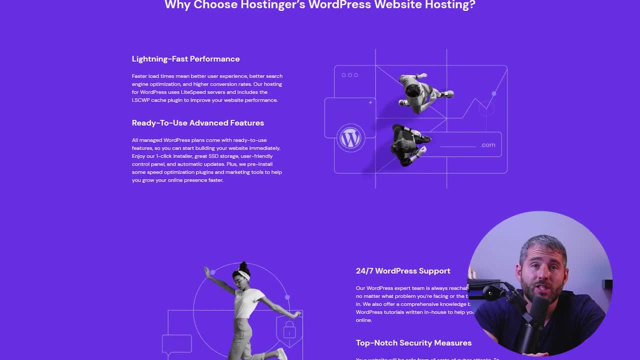 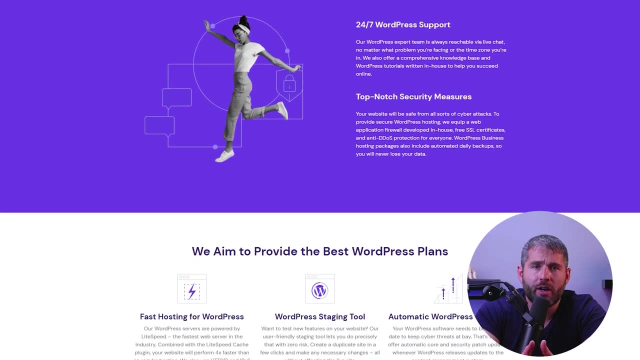 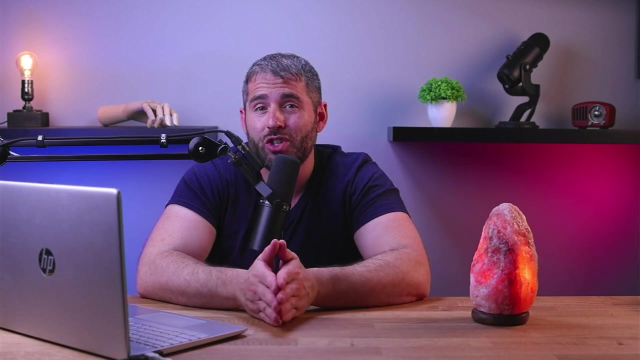 affordable. Lastly, there's WordPress Hosting, which is specifically designed to boost your website's performance and security. if you're using the WordPress Content Management System, Most providers will take care of any WordPress-related updates and technical adjustments, making it a great option for those who want to focus on content creation rather than technical. 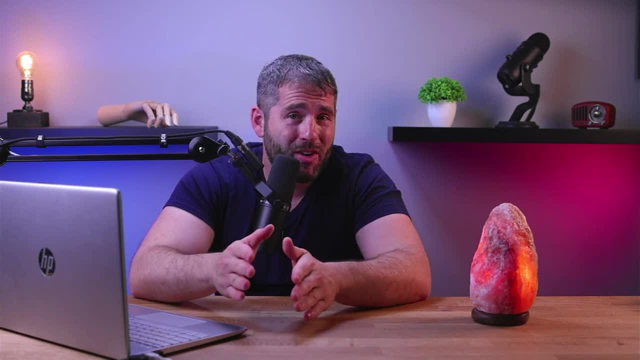 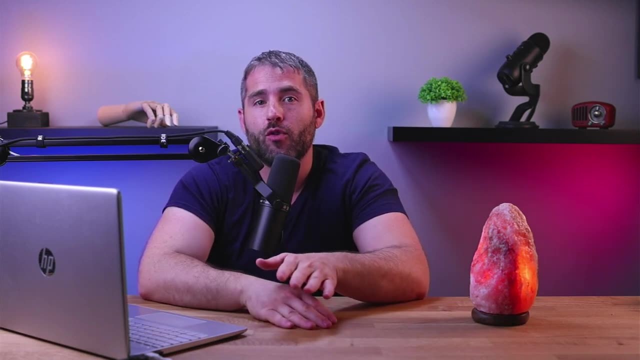 aspects. Now that I've covered the process of picking and comparing services, Here's some additional things to take into consideration throughout your search. When you're creating a website, choosing the right platform and web hosts are crucial for success. The platform you choose will affect how easy it is to create and manage your site, and 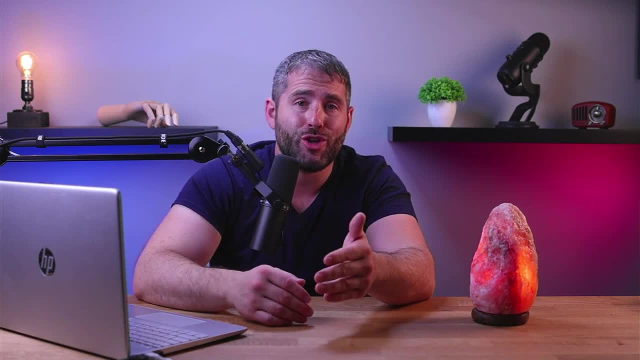 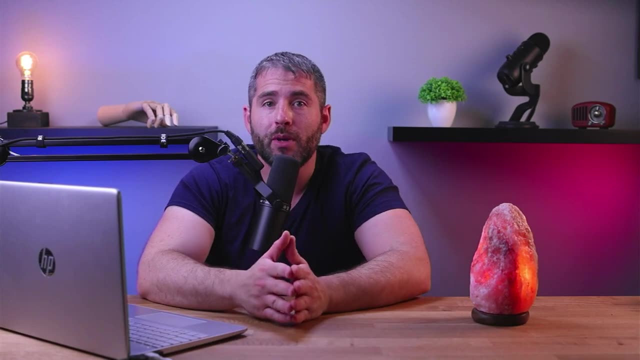 the web host you choose will impact your website's performance, storage and security. Content management systems like WordPress, Joomla and Drupal are popular choices for building websites from scratch, but they require more technical knowledge to manage If you want a simpler option.